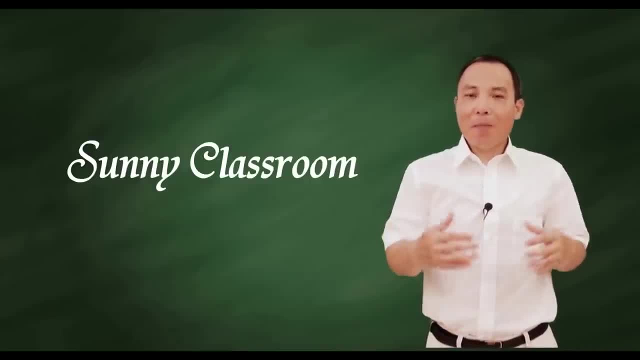 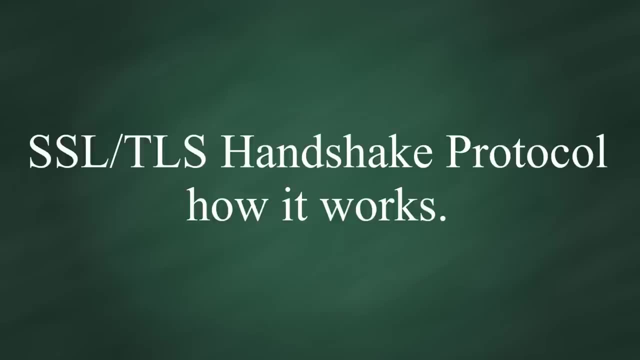 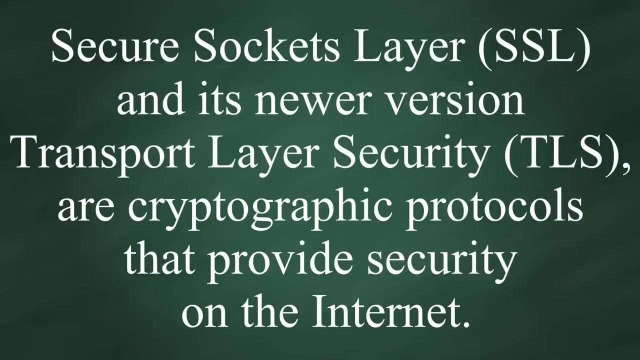 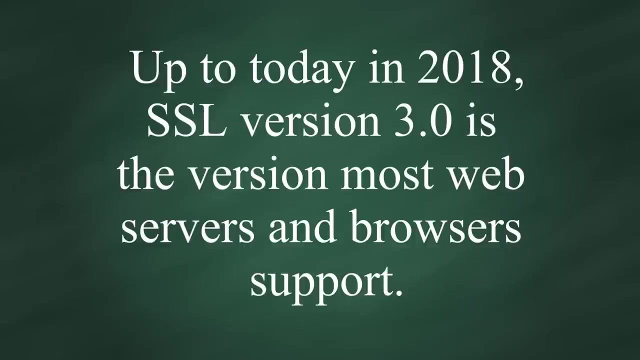 Hello, and this is Sony. Welcome back. Today. my topic is SSL-TLS handshake protocol and how it works. Secure Sockets Layer and its newer version, Transport Layer Security are cryptographic protocols that provide security on the Internet. Up to today, in 2018, SSL version 3.0 is the version most web servers and browsers support. 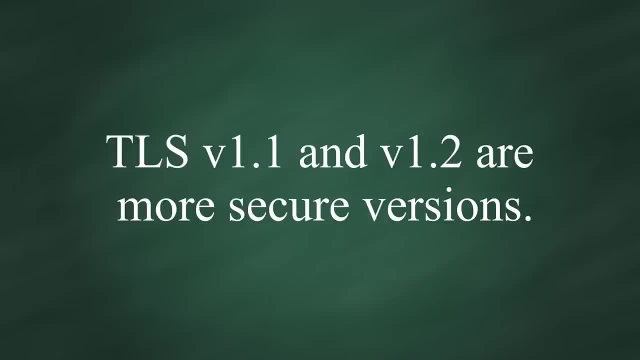 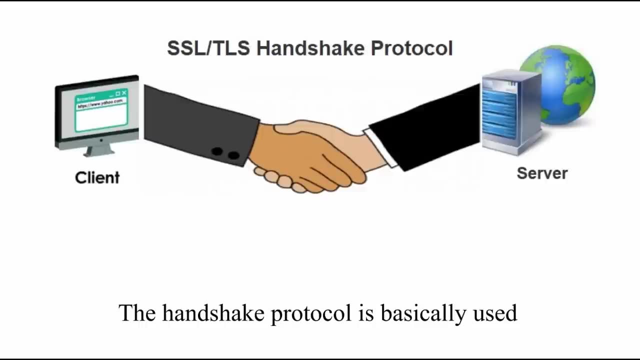 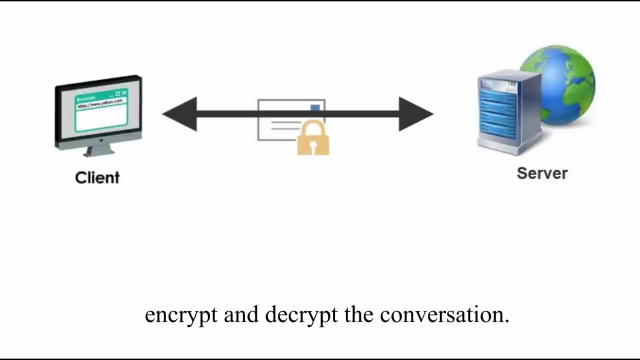 TLS version 1.1 and version 1.2 are more secure versions. The handshake protocol is basically used between a web client and a web server to establish trust and then negotiate what a secret key should be used to encrypt and decrypt the conversation. 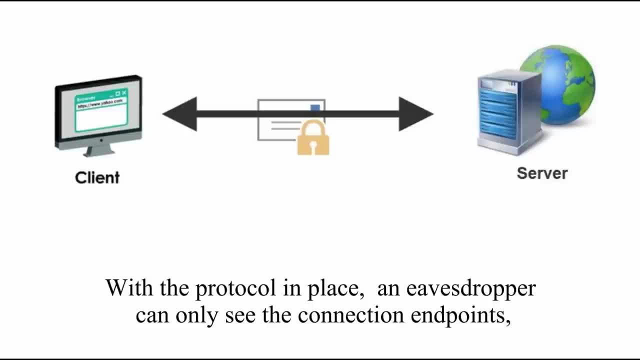 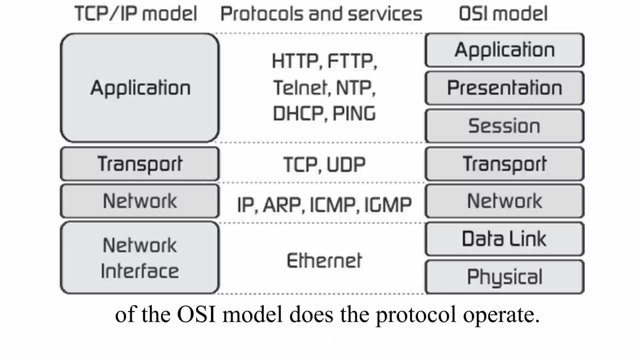 With the protocol in place, an eavesdropper can only see the connection endpoints, but cannot read or modify any of the actual data. Thus, it can protect users' personal data and ensure a safe transaction. Many people are asking: on what layer of OSI model does the protocol operate? 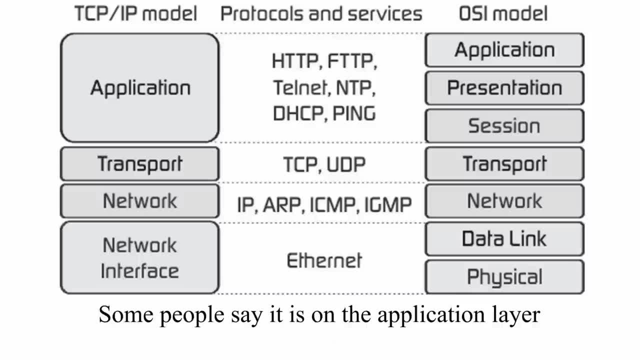 Some people say it is on the application layer because it is just HTTP over secure sockets layer, And some people say it is presentation layer because encryption and decryption operate on this layer. But some argue it is on session layer because the protocol provides point-to-point session security. 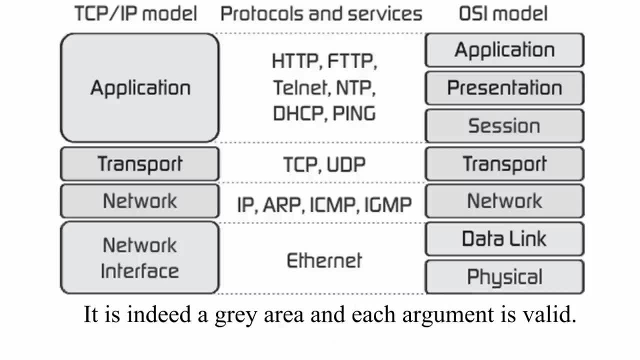 It is indeed a gray area and each argument is valid. The OSI model is not science and is only a guideline. The handshake protocol is involved with the top three layers OSI model And if we use TCP IP model, we can simply say the protocol belongs to the application layer.